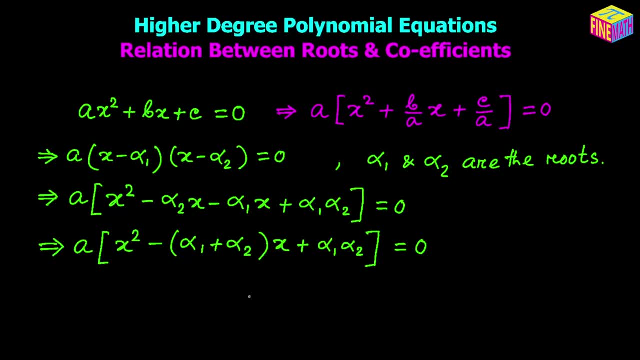 right, because they are the same equation. We just have used the roots in one of the forms and in the other form we are not using the roots, but they are the same equation. So let's compare them and you can see that the coefficient of x 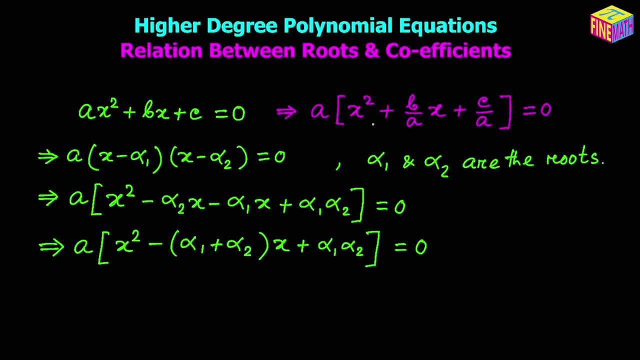 squared is same in both the cases: In the pink form, here the form in the pink color, there the coefficient is one, and in the green color also the coefficient is one. right here, Let me underline: right here, So, or maybe I can simply write that one right here, So. 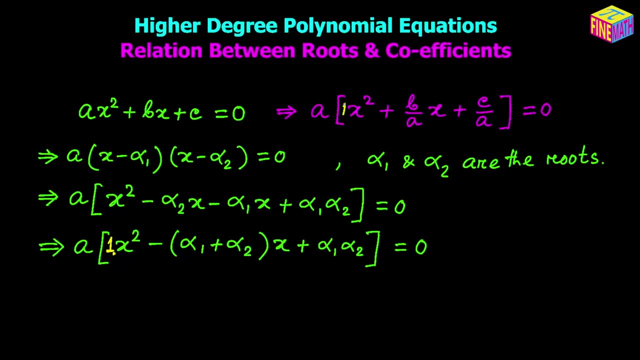 this is the coefficient one times x squared, and here also one times x squared. So the coefficient of x squared is one, And then whatever the coefficient of x squared is the coefficient of x. well, the coefficient of x here is kind of looking like this, If 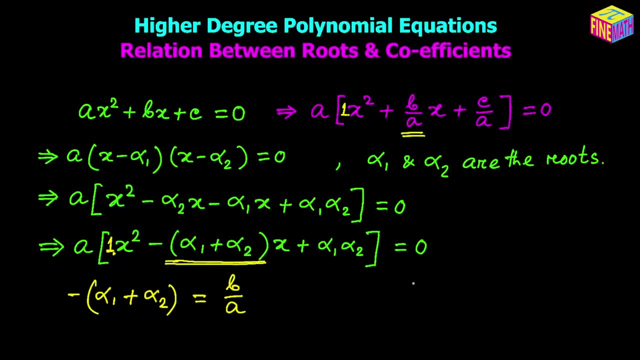 you look at the coefficient of x in both the forms, you will see that in one form we have positive b over a and in the other form we have negative of alpha sub one plus alpha sub two. So they are equal because they are the coefficient of x. So they better be equal. 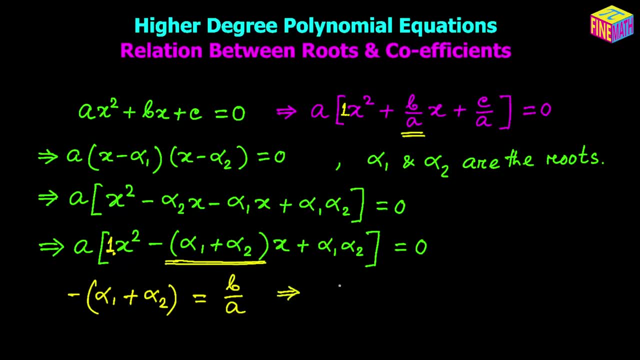 Now, from here, what can you say? Well, from here we can say that alpha sub one plus alpha sub two must be equal to negative b over a. And then, if we compare the constant term between the two forms, if we compare the constant term, how is it going to look like For the? 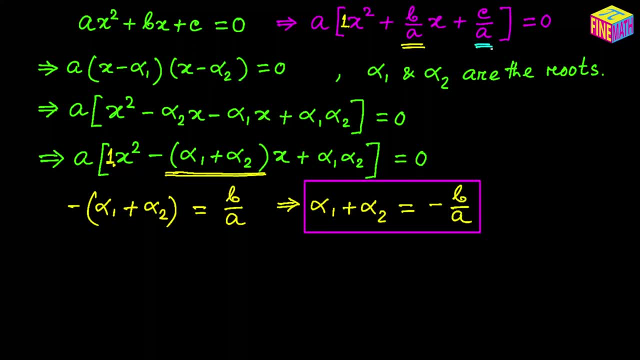 constant term. you can see that in the first form we have positive c over a and in the second form we have alpha sub one times alpha sub two. So I am going to compare those two. They better be equal. So we can say that alpha sub one times alpha sub two, that will be equal. 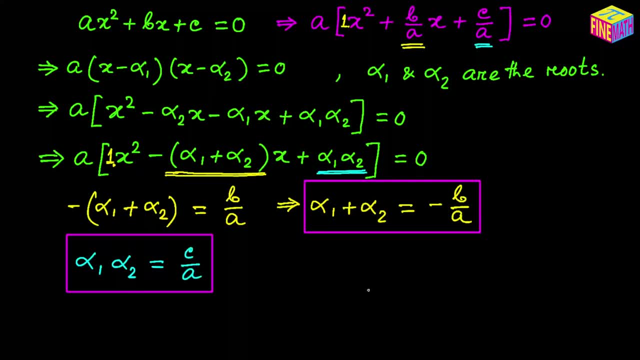 to positive c over a. So for the quadratic equation, we can see that the sum of the roots is actually negative b over a and product of the roots is actually positive c over a. Now what is b? Well, b is the coefficient of the x term, and what is a? a is the leading coefficient. 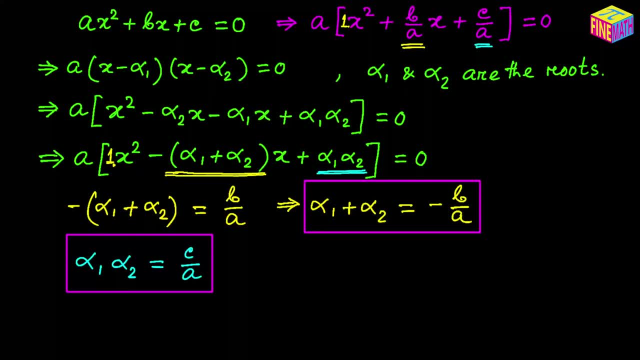 and what is c? c is the constant term, So let me make a quick note here that c is the constant term and a is the leading coefficient. Now let's take a cubic equation and see how this works. Let's suppose we have a cubic equation like this and it can also be written like this. If we take 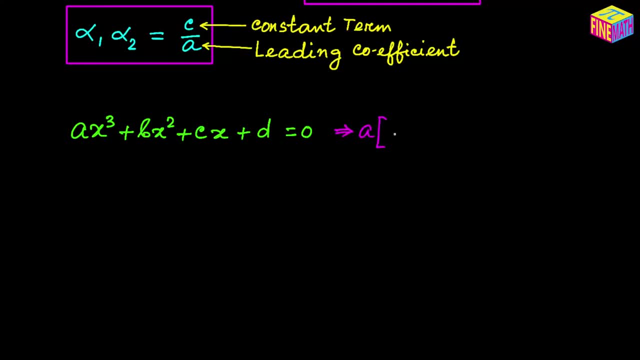 a as a common factor out, then it's going to look like this: Now, if we assume that the three roots of this cubic equation are alpha sub 1 and alpha sub 2 and alpha sub 3, then can we rewrite this equation like this: And now we are going to multiply the three factors together and let's 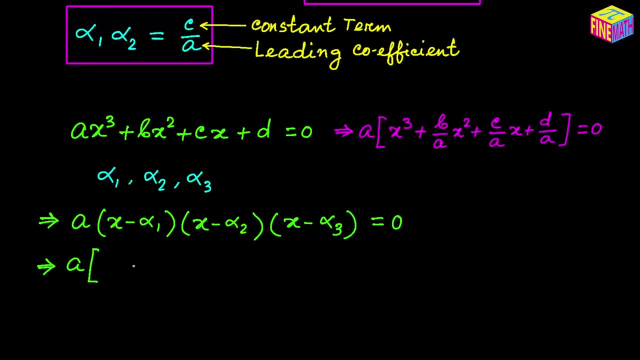 see what happens. First we are going to multiply the first two factors. So, from the first two factors, what are we going to get? We are going to get something like this: and then we have one other factor, which is x minus alpha sub 3, and now we are going to multiply those two factors. the 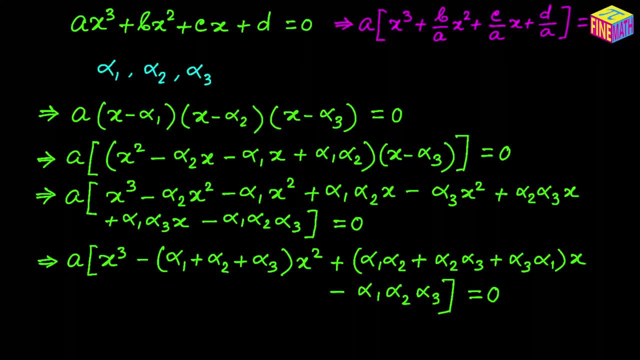 big one and the small one, right? So let's see. So finally, it's going to look like this. It will have a times then: x cubed minus alpha sub 1 plus alpha sub 2 plus alpha sub 3 times x squared plus alpha. 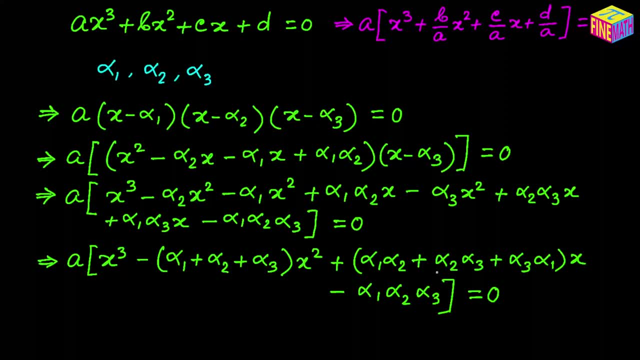 sub 1 times alpha sub 2 plus alpha sub 2 times alpha sub 3, plus alpha sub 3 times alpha sub 1, whole multiplied by x, and then minus alpha sub 1 times alpha sub 2 times alpha sub 3.. All of that is equal to 0. So now our cubic equation kind of looks like this: So now we: 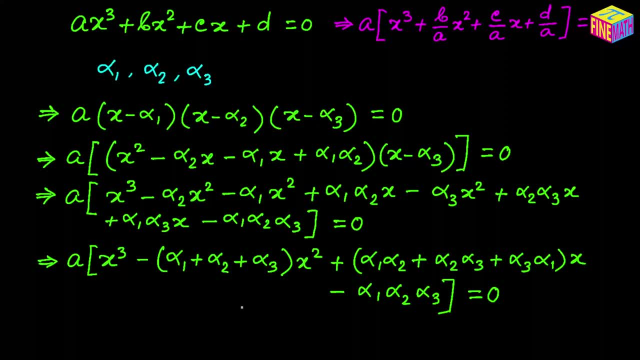 are going to compare the two forms and see how the coefficients match up right. So now, if you look at this coefficient right here, if you look at the coefficient of x squared, in the first form we have positive b over a, but in the second form we have negative sum of the. 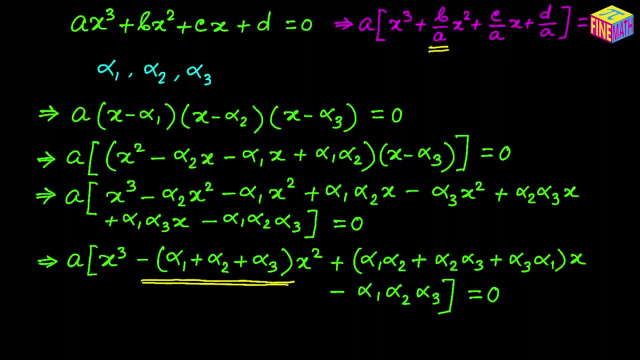 three roots. As you can see right here, it's negative sum of the three roots. So if we compare them, then how is it going to look like? Well then we can say that positive b over a must be equal to the negative sum of the roots. So we can say, well, negative alpha sub 1 plus alpha. sub 2 plus alpha. 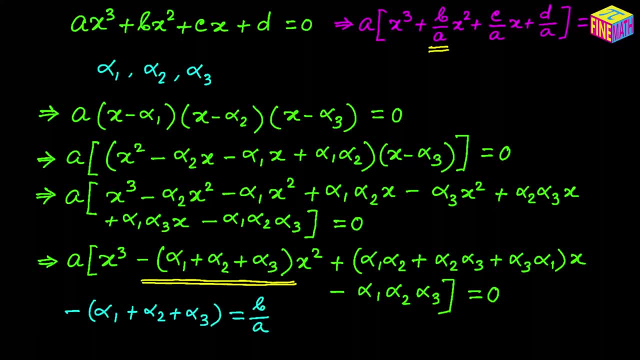 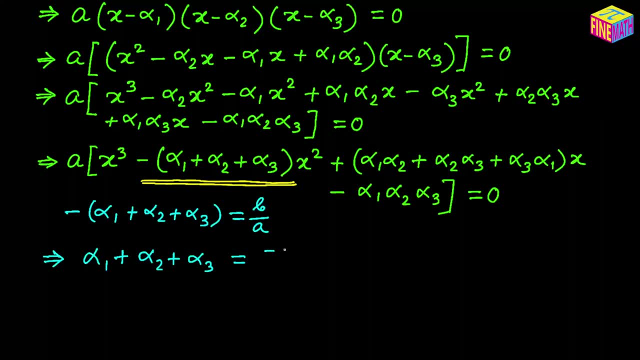 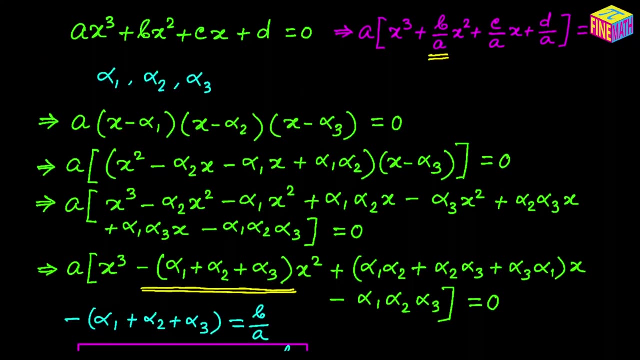 sub 3, that is equal to positive b over a. and then from here we can say that alpha sub 1 plus alpha sub 2 plus alpha sub 3 is equal to negative b over a. and then if we compare the coefficient of the x term, the coefficient is going to kind of look like this In the original equation: we have coefficient. 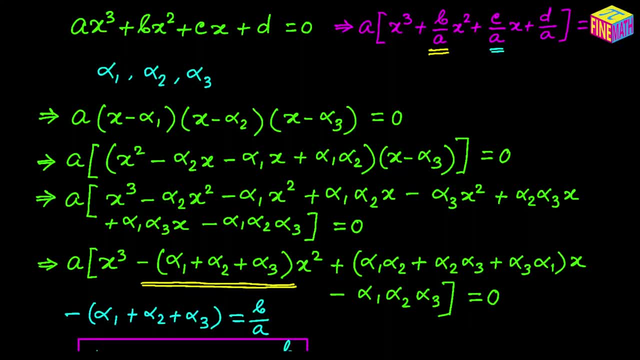 of x term as positive, c over a, and then in our other form, here we have it as positive: the sum of the product of two roots at a time, right. So it is alpha sub 1 times alpha sub 2 plus alpha, sub 2 times alpha sub 3 plus alpha. 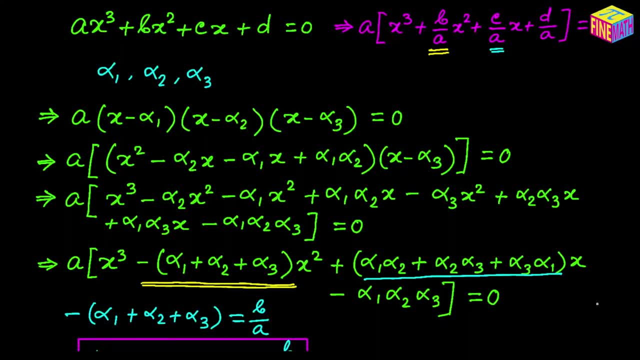 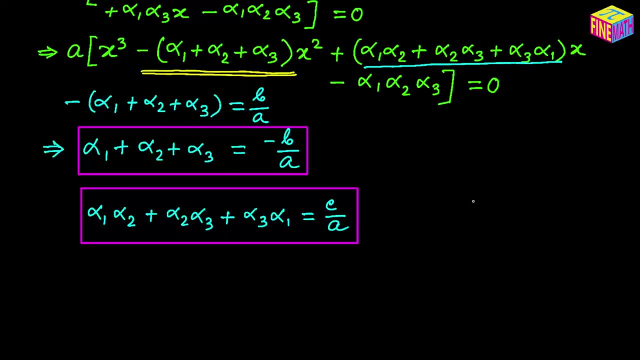 sub 3 times alpha sub 1, so we can compare them then. so then can we write it like this, and this is another important relationship. so I have highlighted that, and now let's compare the constant term in both the forms. so in the first form, what is the constant? 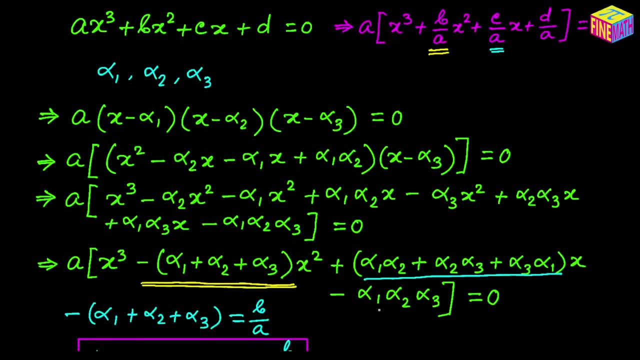 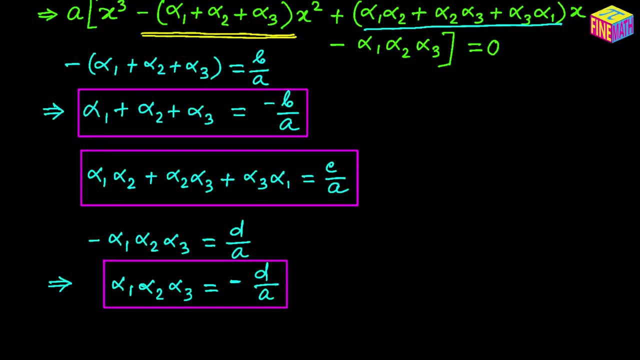 term. in the first from the constant term is positive d over a, and in the second form the constant term is negative alpha sub 1 times alpha sub 2 times alpha sub 3.. So we can compare them just like this, then, and this is the other important relationship between the roots and the coefficients. Now one 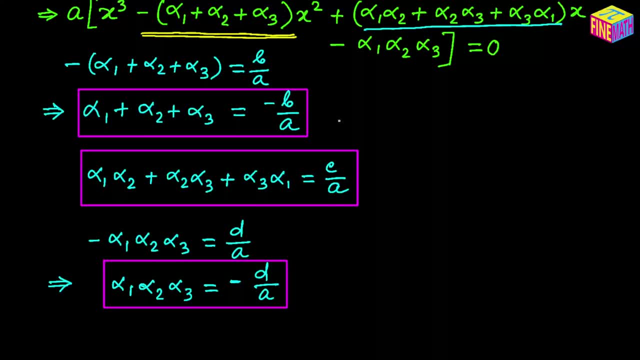 thing to notice here. if you look at the first one right here, where we have the alpha sub 1 plus alpha sub 2 plus alpha sub 3, that is equal to negative b over a. can we write this as negative 1 whole to the power 1 times b over a? and then over here on the second one where we have the alpha sub 1 times? 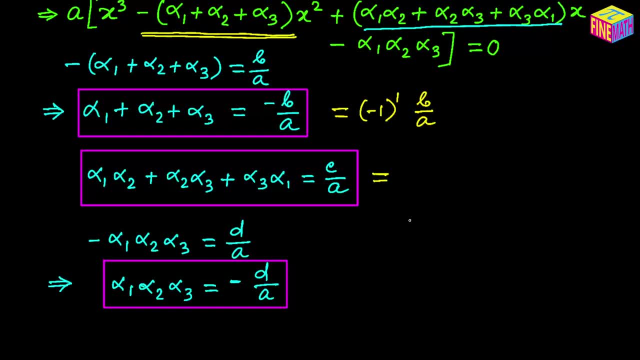 alpha sub 2 plus alpha sub 2 times alpha sub 3 plus alpha sub 3 times alpha sub 1 equals positive c over a. can we write that as negative 1 squared times c over a? think about it, because negative 1 squared would be positive 1, and that's exactly what we have: positive c over a. and then in the 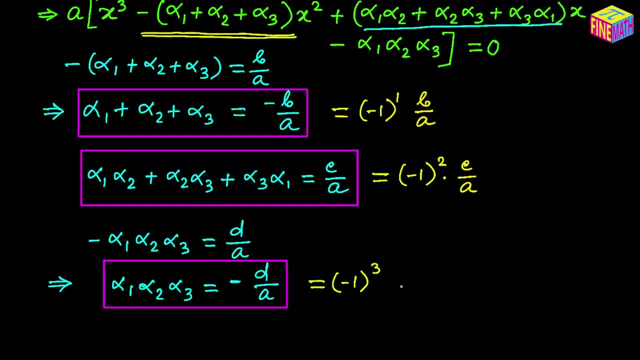 third one, can we write it as negative: 1 cubed times d over a. so you are starting to see a pattern here, right? the pattern is that as we take higher and higher degree polynomial, we are going to see the relationship between the roots and the coefficients, which kind of going to go like this: 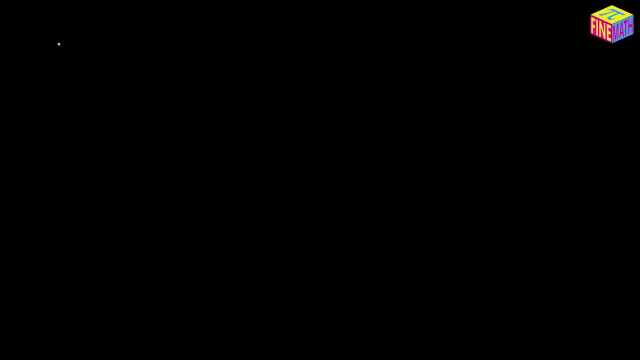 next, let's take a quartic equation and see how this works out. let's suppose we have a quartic equation like this: if we take out a as a common factor, can we rewrite the equation like this: now let's assume that the roots of this quartic equation are alpha sub 1, alpha sub 2, alpha sub 3 and alpha sub 4.. So, using 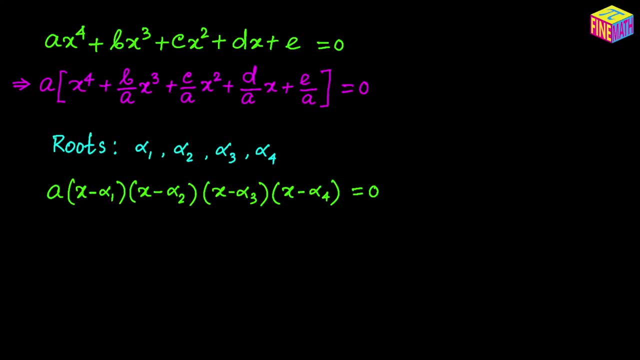 the factor form. can we rewrite the equation like this: now let's try to multiply the factors one by one. so first we are going to multiply the first two factors, and then the equation is going to look like this: the product of the first two factors would look like this, and then we have 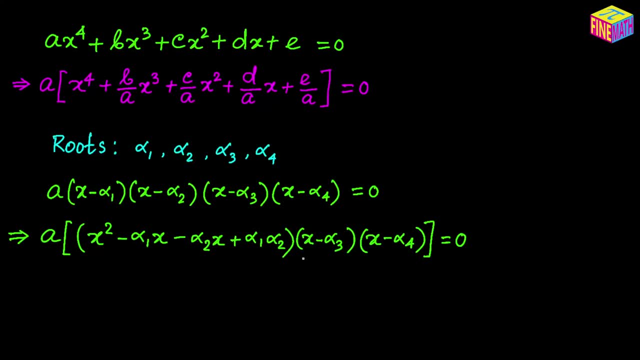 factors. Now let's try to multiply the bigger factor with the next smaller factor, and then, finally, we are going to multiply the last factor with the large factor here, right? So let's do that multiplication. Now let's try to group the like terms together. First we are going to write: 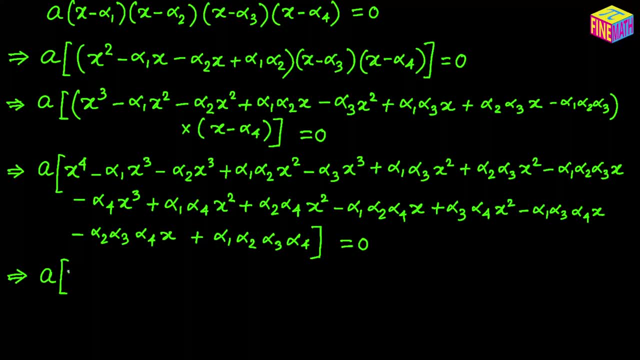 the x to the power 4 term as is. We only have one term here, which is x to the power 4. and then let's try to group the x cubed terms. Actually, we have four of them, So we can write it like this and: 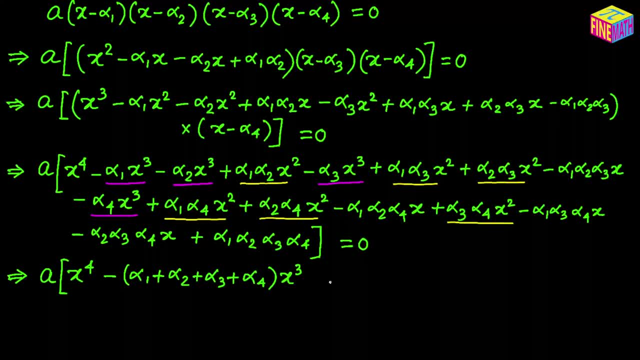 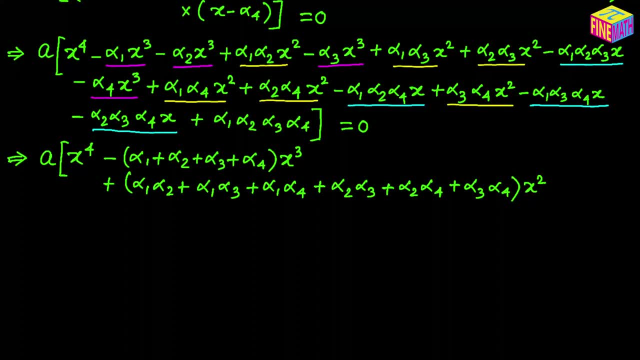 then let's try to group the x squared terms. We have six of them, and we can group them like this. and then let's group the x terms. We have four of the x terms, so we can group them like this. and finally, we have the constant term, which is alpha sub 1 times alpha- sub 2 times alpha. 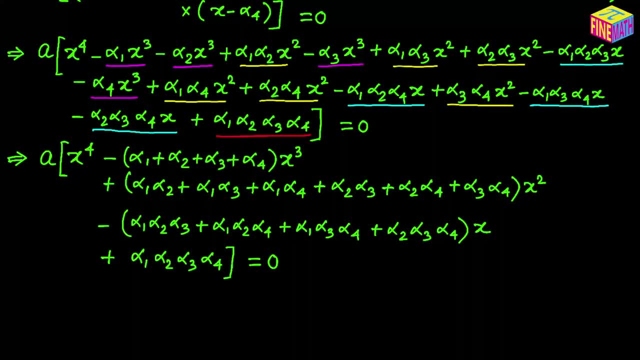 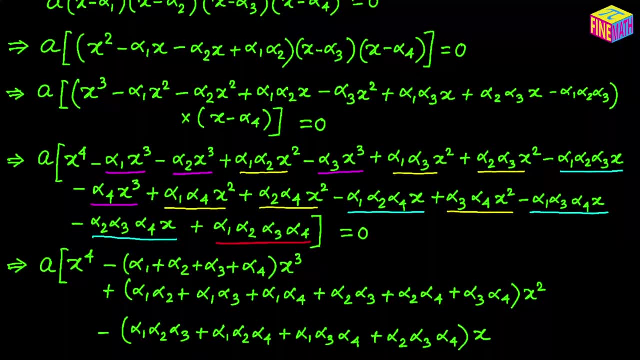 sub 3 times alpha, sub 4.. Next, we are going to compare the coefficients of these various terms with the original form that we had up there. So let me scroll up little bit and you see that original form in the pink color We are going to 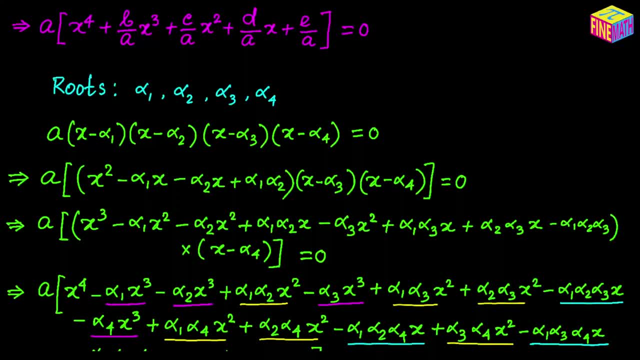 compare the coefficient of these various terms, like, for example: you know, we'll be comparing the coefficient of x cubed term and then we'll be comparing the coefficient of x squared term, then the x term and the constant term. right, So let's do that comparison. I'm going to write down this pink color form once: 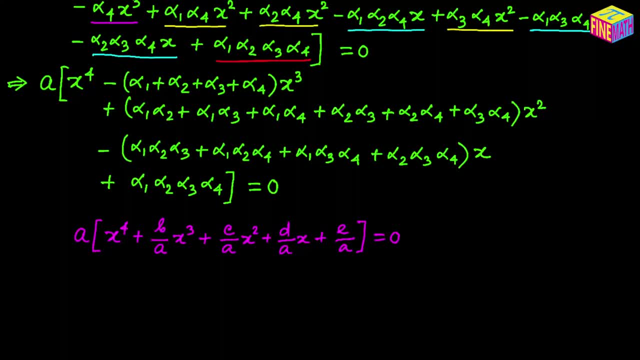 again down below, If you look at the x to the power 4 term, they both have the coefficient as 1.. There is no coefficient means there is a coefficient 1. So there is really nothing to compare. Now, if you look at the x cubed term between these, 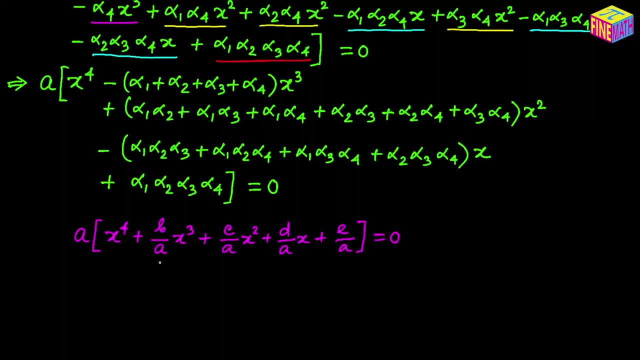 two forms you will see. in the original form we have b over a as the coefficient of x cubed term. but in the new expanded form we have alpha sub 1 plus alpha sub 2 plus alpha sub 3 plus alpha sub 4 and their negative value, that is the. 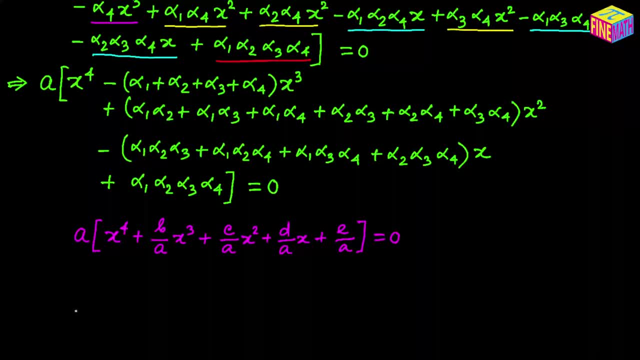 coefficient of x cubed term. right, So can we compare it like this? So, comparing the coefficient of the x cubed terms, we can write it like this: and if we multiply both sides by a negative 1, we are going to get something like this and we can. 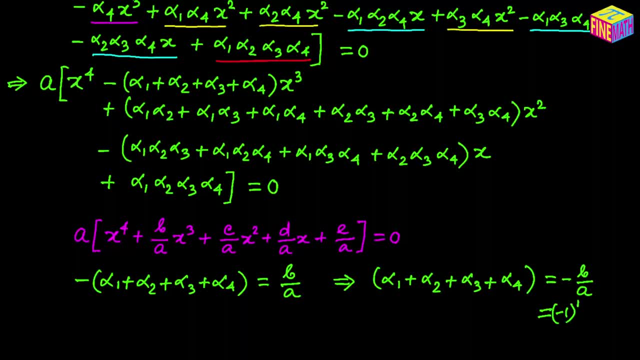 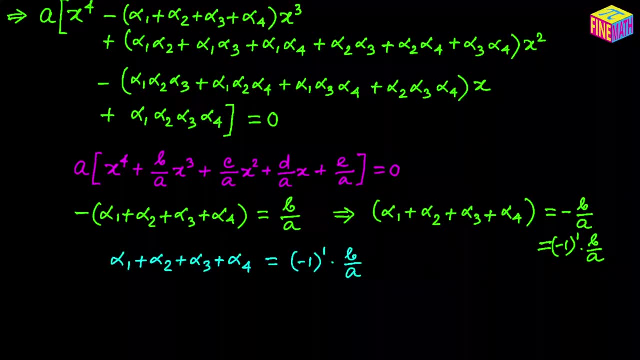 also write it like this: We can say negative 1 with a power 1 or exponent 1 times b over a, So finally we get something like this. Now, in this case, what is b? Well, b is the coefficient of the x cubed term. 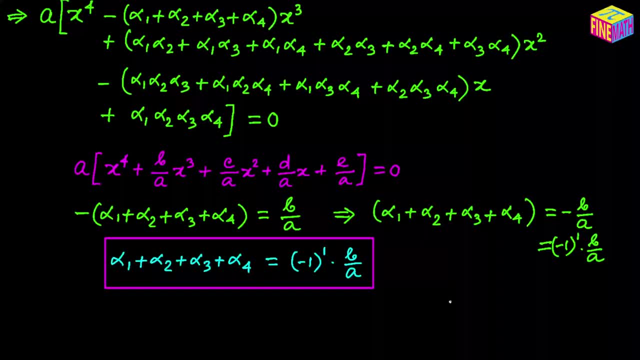 and a is the leading coefficient. right Now let's compare the coefficients of the x squared terms. In the expanded form, the coefficient of the x squared term is like this, and that will be equal to c over a, because that is the coefficient of the x squared term in the original form and that can be written as negative 1 squared. 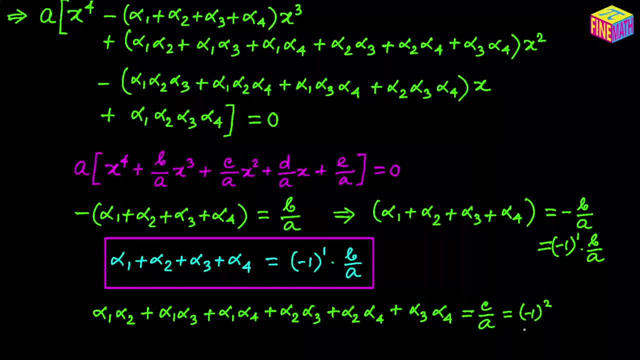 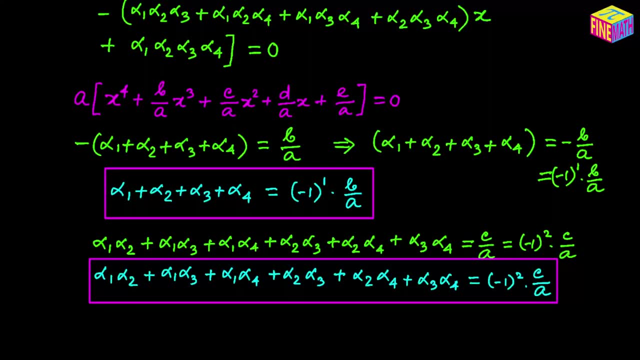 because we have a positive c over a right. So we are intentionally writing it like this to establish a pattern here. So this will be negative 1 squared times c over a. So finally we get something like this. So this is another important relationship between the coefficients and the roots of the equation. Now let's 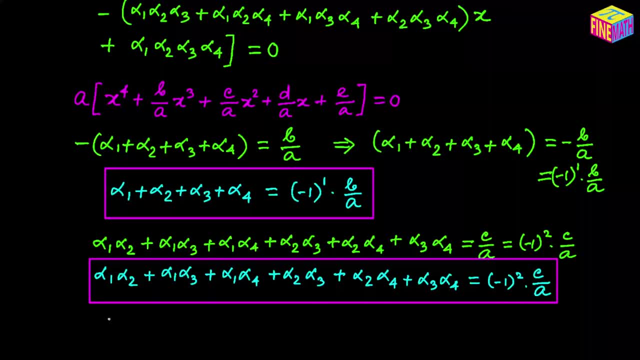 try to compare the coefficients of the x terms. In the expanded form, the coefficient of the x term is like this, and that will be equal to positive d over a, because that is the coefficient of the x term in the original form. Now if we both sides by a negative 1, then it's going to look like this. That will be. 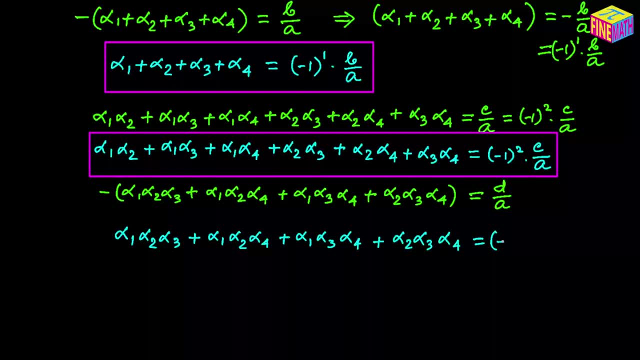 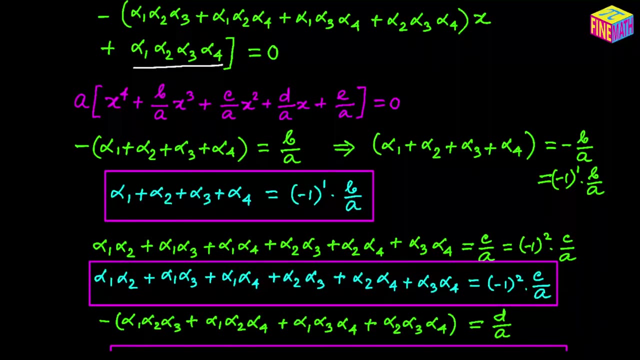 equal to negative d over a, and for that negative I am going to write it like this: and that is our other relationship between the coefficients and the roots. And finally, we are going to compare the constant terms. In the expanded form, the constant term is like this: I am doing a white underline here, which is alpha sub. 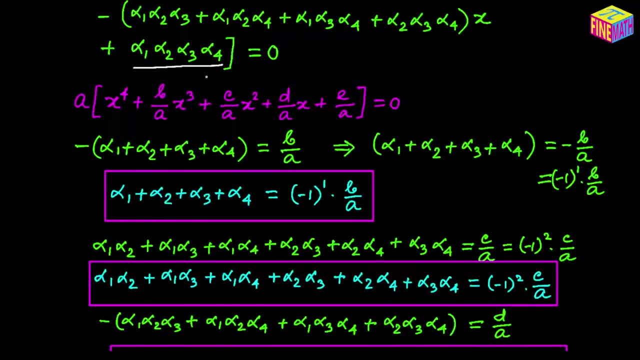 1 times alpha sub 2 times alpha sub 3 times alpha sub 4.. That is the constant term. and then in the original expression the constant term is actually e over a, So I do another white underline there. So now let's compare those two. So that is. 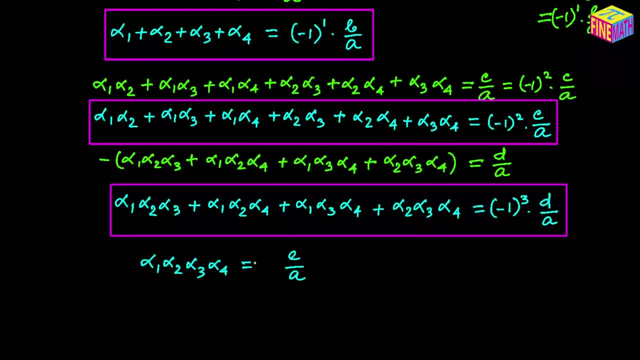 positive e over a and I am going to intentionally write it like this: Negative 1 power 4 times e over a. and that is our last important relationship between the coefficients and the roots. And finally, we are going to take a polynomial equation and we are going to try and establish the relationship. 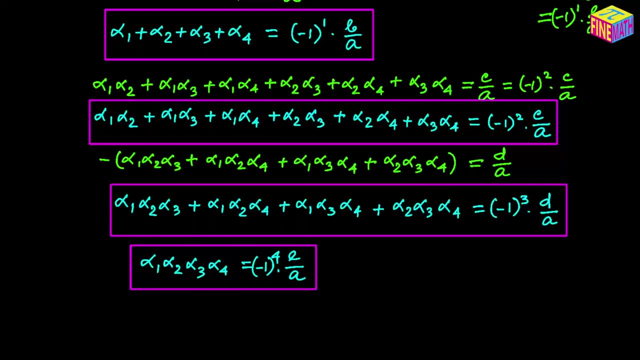 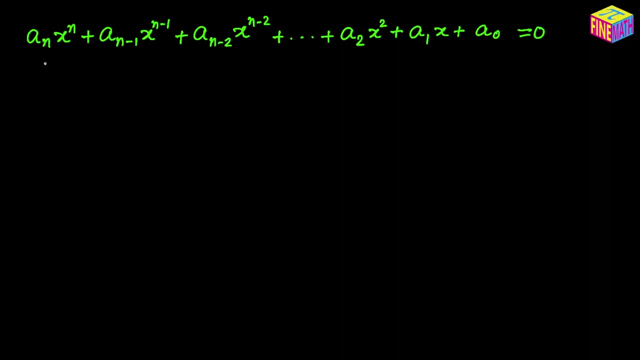 between the coefficients and the roots. So let's take a generic polynomial equation of n degree. Let's suppose this is our generic polynomial equation of n degree. and now if we take the leading coefficient out as a common factor, then this equation can be rewritten like this. Now let's 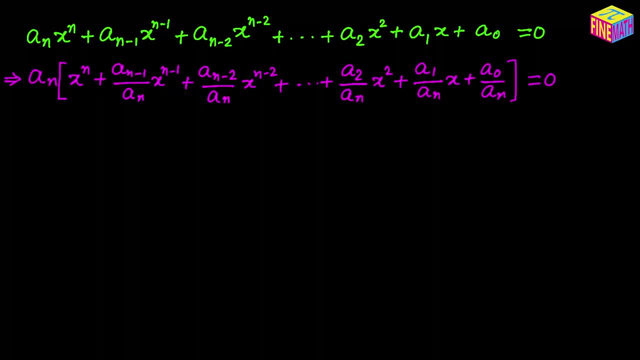 assume that the n roots of this n degree polynomial equation are like this: Let's assume that the roots are alpha sub 1, alpha sub 2, alpha sub 3, etc. up to alpha sub n, and there will be n roots because the degree of this polynomial equation 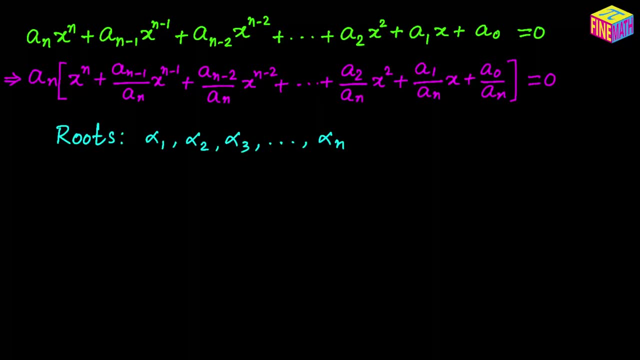 is n, So there will definitely be n roots. Now, using the factor form, can we rewrite this equation like this: And there will be total n such factors. I mean other than the leading coefficient, of course. And now, if we multiply all of them together and try to expand this, 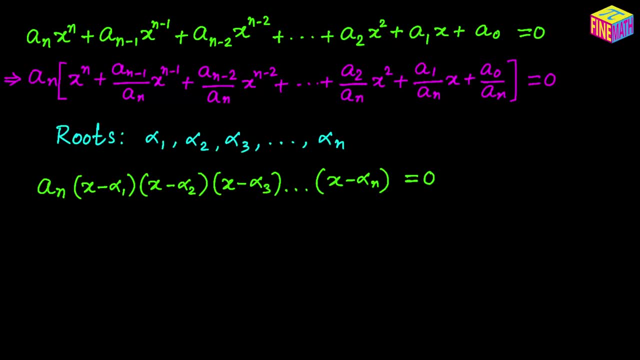 form. it is going to follow the same pattern that we have seen for a quadratic or a cubic or a quartic equation. right, I am not going to try and expand because we really don't know what is the value of n, So we really cannot. 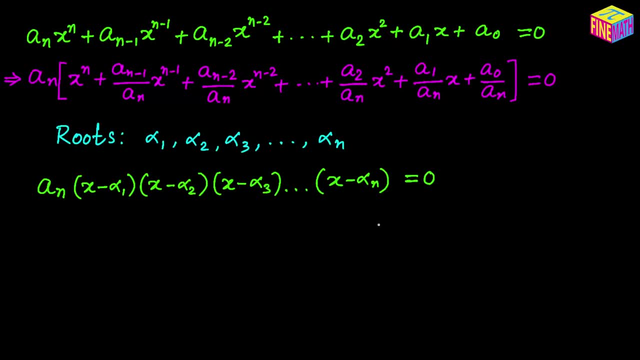 try and expand it like this, But I can show you what is the pattern going to be. As you have seen before, the coefficient of the x to the power n minus 1 term is going to be like this: It will pretty much be the sum of the roots kind. 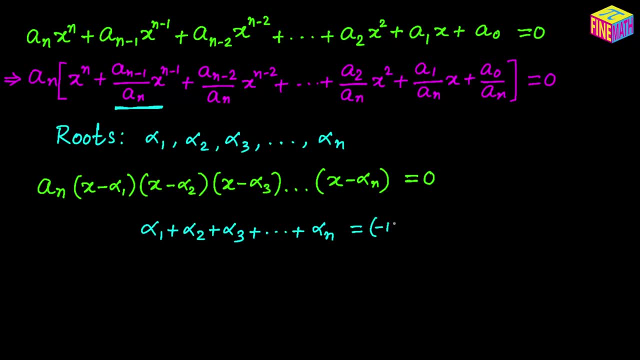 of like this: And that will be equal to negative 1 to the power, 1 times the coefficient of the x to the power n minus 1 term in our original form. right there I have underlined that term right there. So that would be a sub n minus 1. 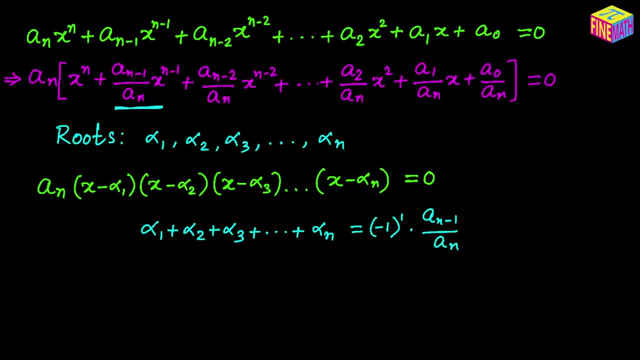 over a sub n. a sub n is the leading coefficient. a sub n minus 1 is the coefficient of the x to the power. n minus 1 term in our original form. But in that form we have a sub n minus 1 over a sub n as the coefficient of x to the 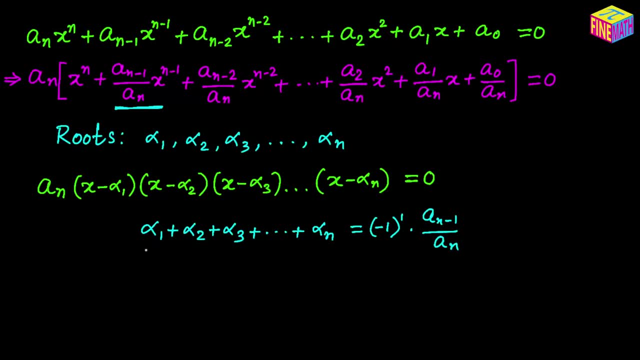 power n minus 1.. And that coefficient will be equal to the sum of the roots, like this, But of course it will be a negative value. So we are keeping the negative 1 to the power 1 on the right hand side, And also this is generally. 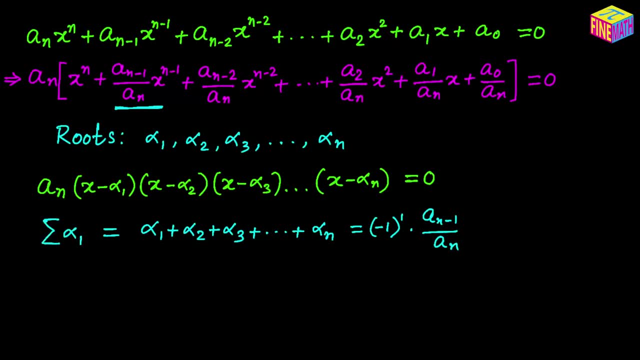 denoted in the Sigma notation like this. And that is a very important relationship between the roots and the coefficients. So let me highlight it Now. if we think about the coefficient of the x to the power n minus 2 term, then in the standard form it would look something like this: And this sum will be equal to: 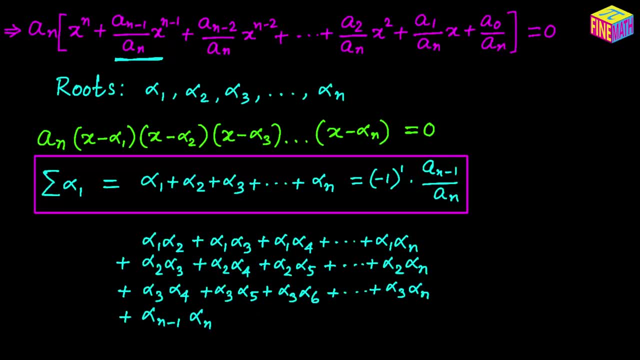 the coefficient of the x to the power n minus 2 term in our modified original equation. And for the positive value, I am going to write it like this: I am going to say negative 1 squared And the coefficient, there is actually a sub n. 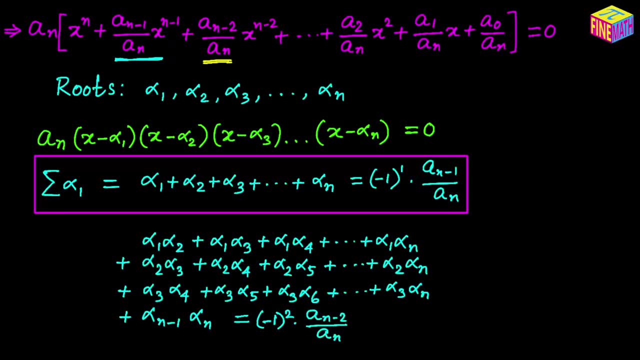 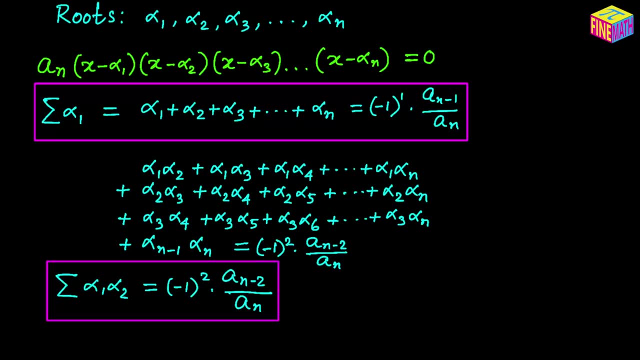 minus 2 over a sub n. Using the Sigma notation it can be written like this: And that is another important relationship between the roots and the coefficients. And similarly, if you think about the coefficient of the x to the power, n minus 3 term. in the original form and the expanded form they're going to be: 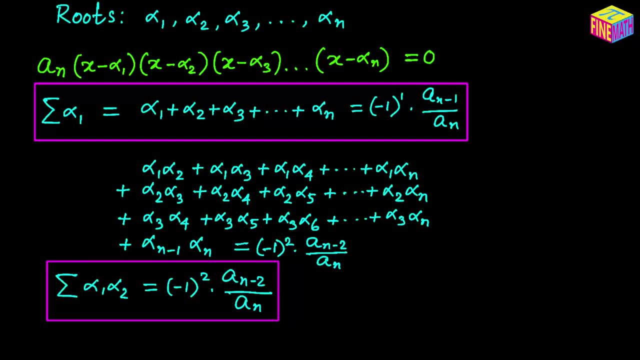 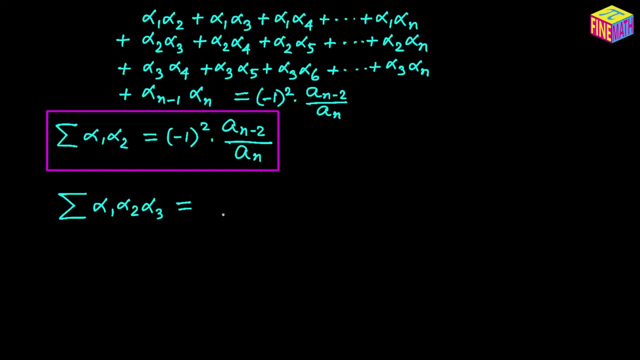 like this: It will be sum of three roots at a time, right, All possible combination of three roots at a time. So we can write it like this and it will be a negative value. It will be negative of a sub n minus 3 over a sub n. So for the 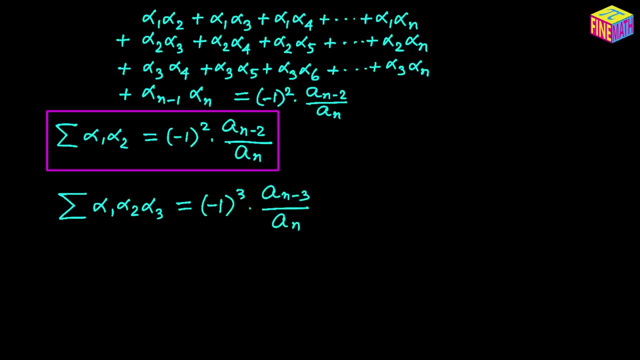 negative. I am going to write it like this, And that is also another important relationship. and similarly, if you think about the coefficient of the x to the power n minus 4 term, they are going to compare kind of Wool trafficking type terms is also another. but 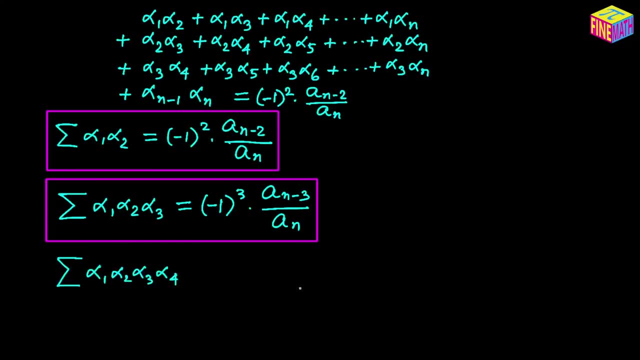 meaningful yesterday and similarly, if you think about the for the x to the power n minus 4 term, they are going like this: it will be the sum of all possible combinations of four roots multiplied at a time, and it will be a positive value. i am going to write it as negative: 1 to the power 4 and it. 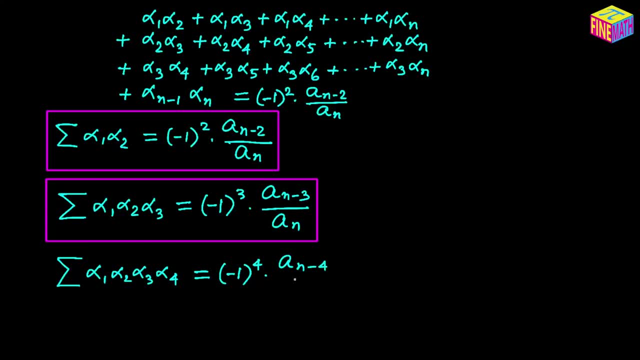 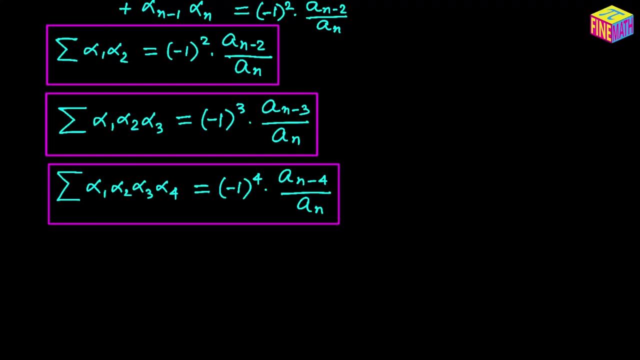 will compare with a sub n minus 4 over a sub n, and that is also another important relationship, and it will go on like this. finally, we are going to see what is the constant term going to look like. for the constant term, it will be the product of all of the roots, so we really do not need to. 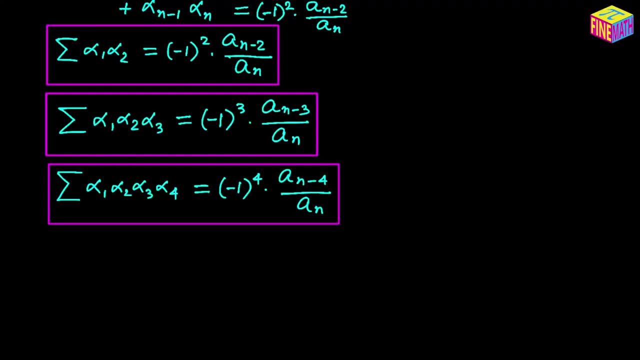 use any sigma notation because it's just a single product and the product is like this: alpha sub 1 times alpha, sub 2 times alpha, sub 3 times, etc. times alpha sub n. so it is just a single product of all of the roots together and that will be equal to negative 1 to the power n depending. 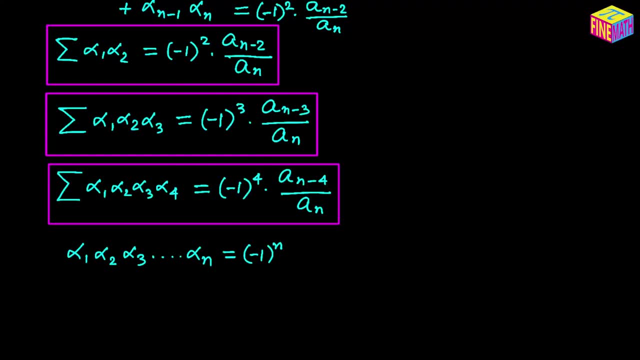 on the value of n. it could be a positive value or a negative value, depending on what is. that n is right and it will be a sub 0 over a sub n. in my example, i have taken a sub n as the leading coefficient, but some authors- or maybe many authors- they- use a sub 0 as the leading. 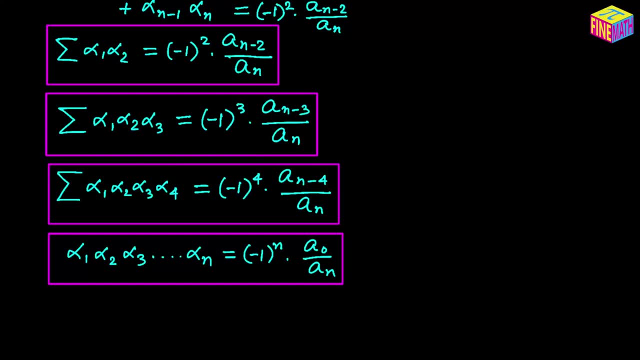 coefficient. personally, i find that a bit confusing, because i would really love to have the same kind of notation for the coefficient as well as the exponent of x. so because the first term is x to the power n, i would prefer to have the leading coefficient as a sub n. that way it's easy to follow. 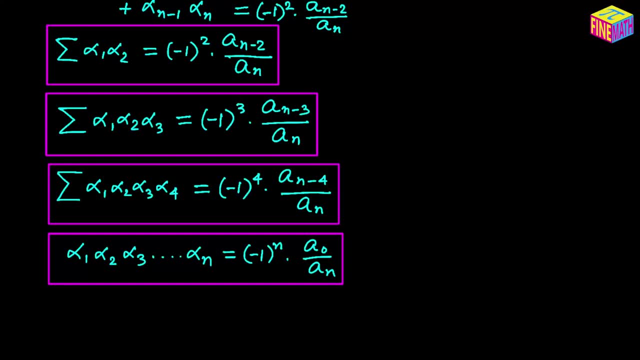 for me. so please keep a note that this, a sub n, is nothing but the leading coefficient. let me kind of write it here. and what is a sub 0? well, a sub 0 is the constant term in our original polynomial equation. now let's take an example and see how we can utilize this concept to solve different. 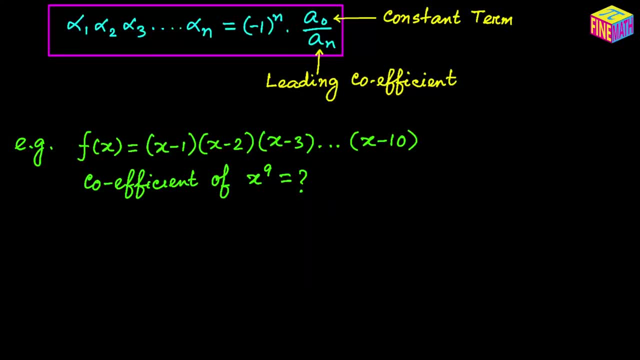 problems right. so i'm going to take an example here. let's suppose we have an example like this, where we have been given that f of x is equal to x minus 1 times x minus 2 times x minus 3, etc. up to x minus 10.. so this is pretty much a factor form of a polynomial expression here, it's not an equation. 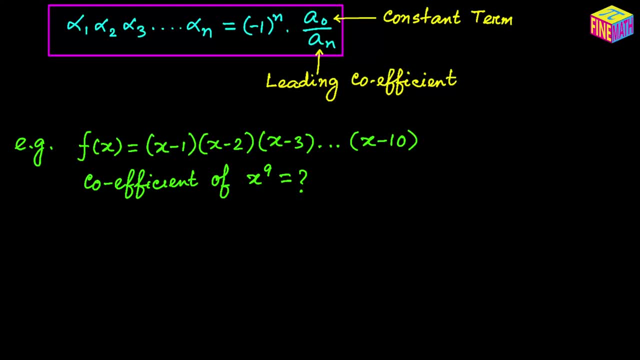 it is a polynomial expression or function, and the question here is that if we expand this function, what would be the coefficient of x to the power 9.. now, from here, clearly you can see that the leading coefficient is 1, so the coefficient of x to the power 10 will be 1.. there is no doubt about that. 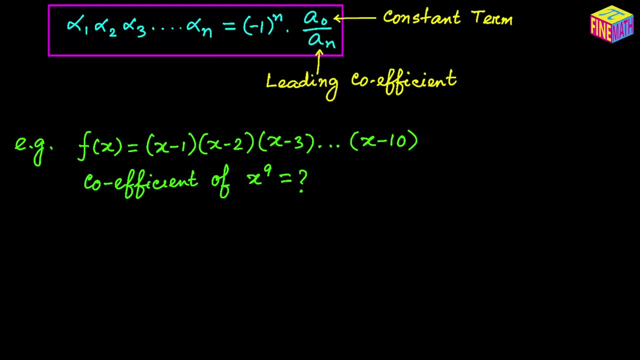 but we have to find out what is the coefficient of x to the power 9 in the expanded form right now. if you sit down and try to expand this thing, it will take some time to do that now. instead of that, what we are going to do, well, coefficient of x to the power 9 is actually going to be some. 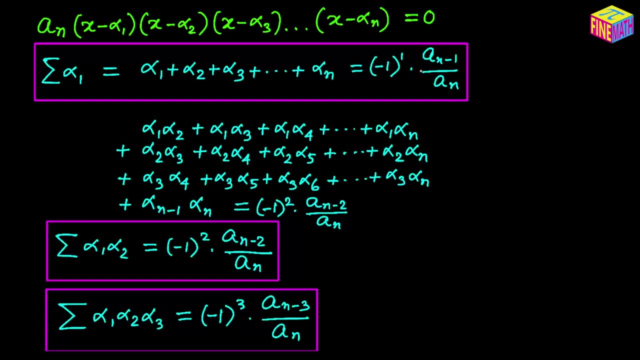 thing like this: coefficient of x to the power 9 will be actually negative: 1 to the power, 1 times a sub n minus 1 over a sub n. now what is a sub n? that's the leading coefficient, and in our example the leading coefficient is actually 1.. so then we have to find out what is the value of a. 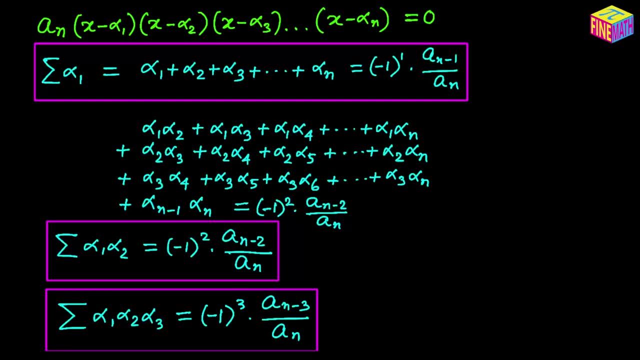 sub n minus 1, and we can easily utilize this particular formula right here. let me kind of highlight it like this: this particular formula, that's what we are going to use- that alpha sub 1 plus alpha sub 2, plus alpha sub 3, all the way up to plus alpha sub n, that would be equal to: 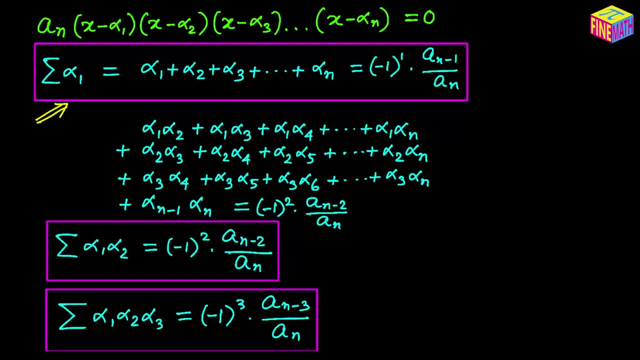 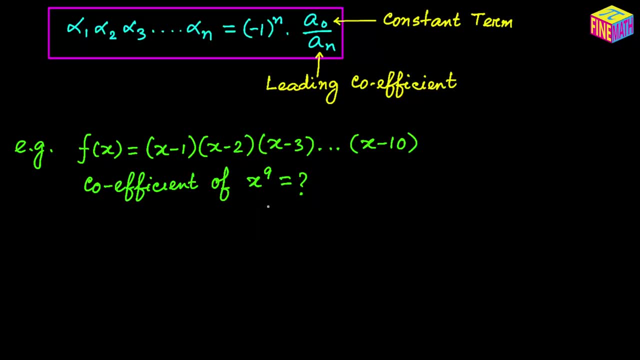 negative 1 power 1 times a sub n minus 1 over a sub n. so using that formula we are going to solve our example very easily. let's try that. so the coefficient of x to the power 9, this is essentially a sub n minus 1, that's the coefficient of x to the power 9, where n is equal to 10. we have been 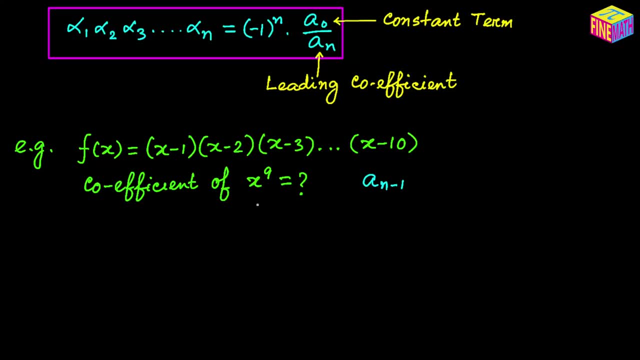 provided a 10 degree polynomial function and we have to find out the coefficient of x to the power 9, which will be essentially a sub n minus 1. and by the way, also, as you can see from the definition of the function, we have a sub n. the leading coefficient is actually 1 because there is 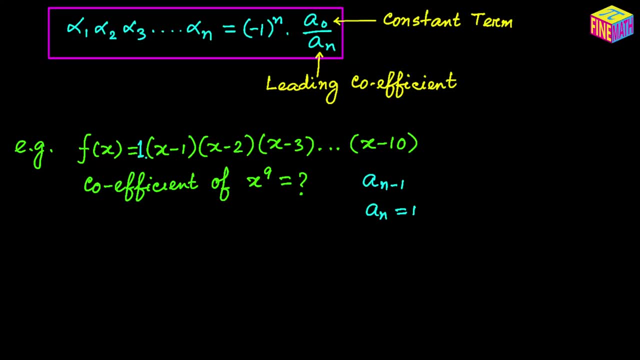 nothing right here, so i am assuming that we have a 1 right there. so our leading coefficient is 1. that means a sub n is equal to 1 and we have to find out what is a sub n minus 1. now. using our formula, we know that negative 1 to the power 1 times a sub n minus 1 over a sub n is.